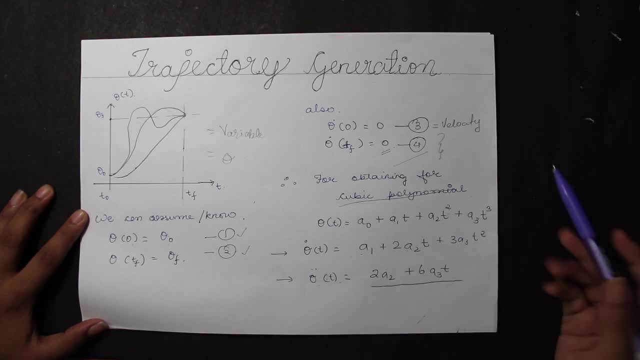 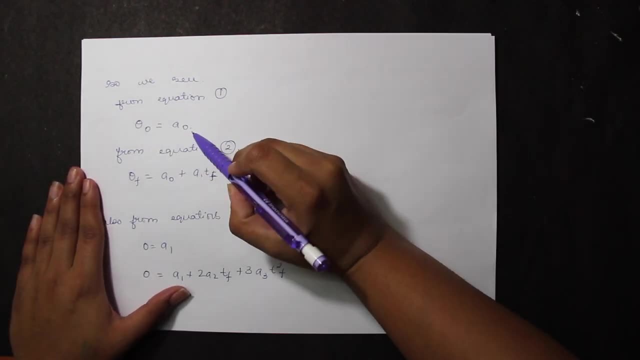 That is 2A2 plus 6A3t. So we see from the first equation, that is of theta naught, of 0 equals to theta naught. We simply substitute the value of t, That is t equals to 0, and we come up to something like this: 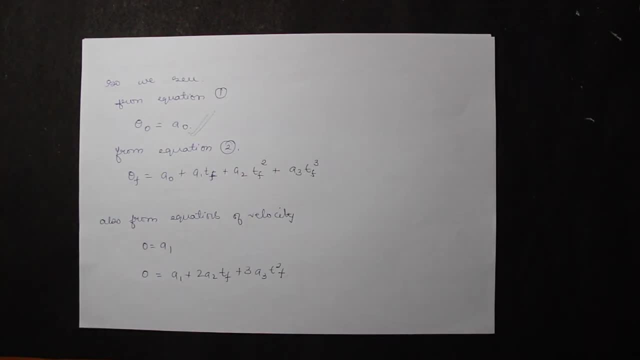 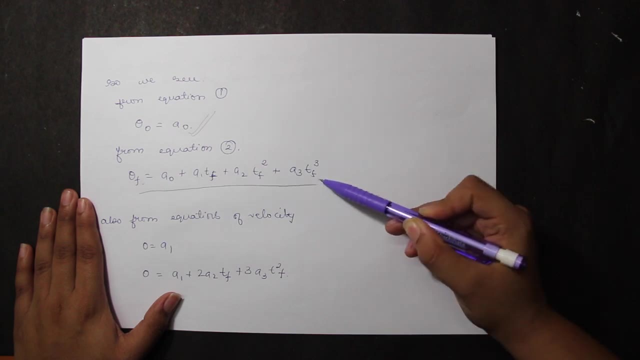 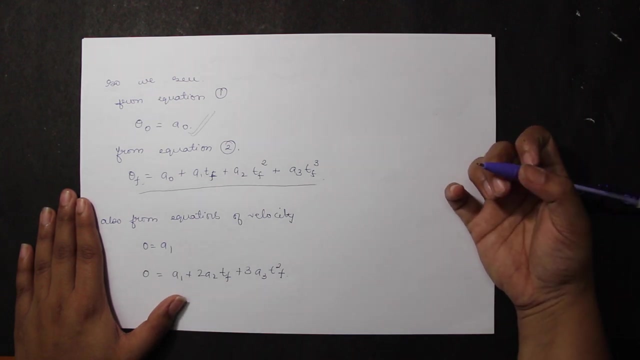 From the final position, that is, the value of theta. theta f at tf will be simply substituting the value of t as tf And we come up to something like this, Also from the equations of the velocities, that is, theta naught dot equals to 0.. 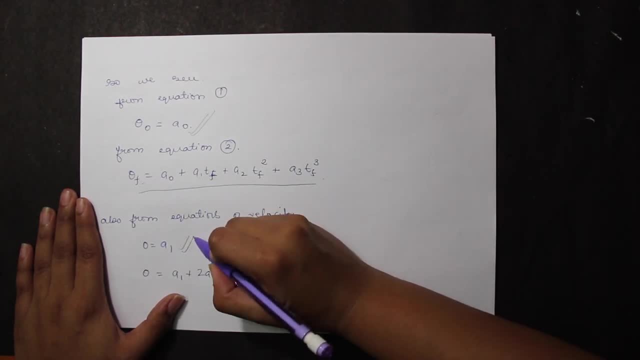 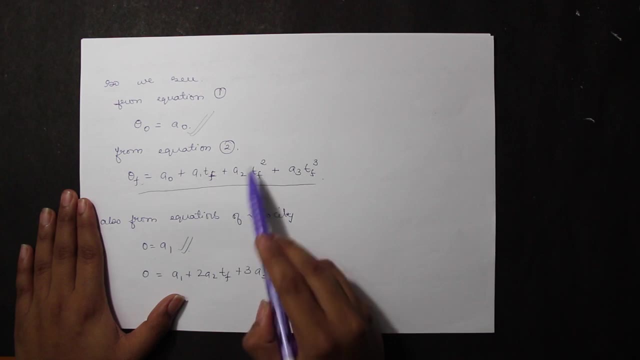 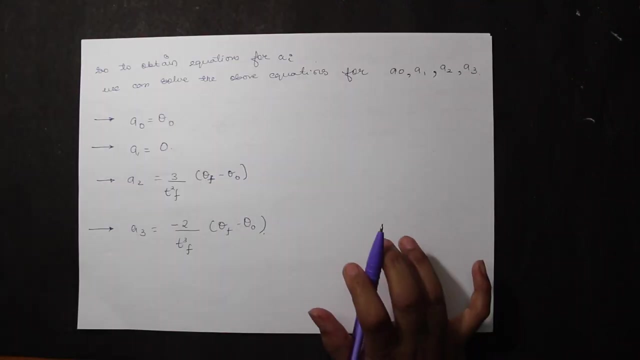 We put it to the value of theta, t, dot, and we come up to something like: A1 will be always 0. When we put the value of tf, we come up to this equation. Okay, now let's derive further, So to obtain the equations of Ai, that is A naught- A1, A2, A3.. 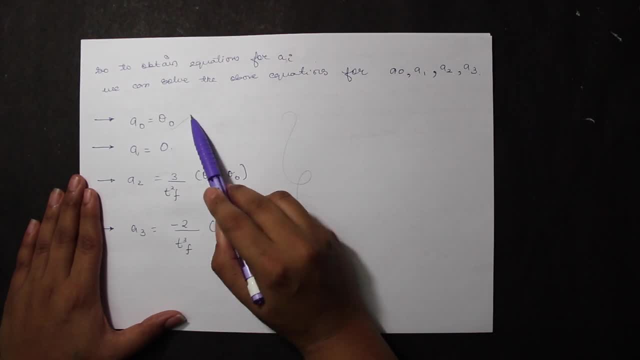 We know the value of A naught is equal to theta naught, since we derived it from the first and the third equation. Similarly, we also know the value of A1 equals to 0. Since we know the velocities At the final position and the initial position is 0, and I just explain you like two minutes back. 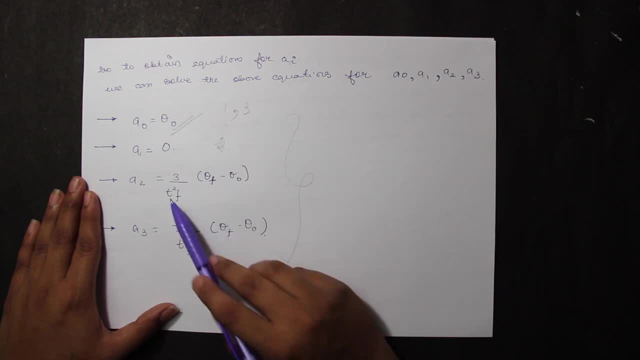 Here we have to find the value of A2 and A3. You can find out that by solving the equations We have initially derived, that is, from equations 4 and 6.. Similarly, we find out the value of A3 from the fourth and the sixth equations. 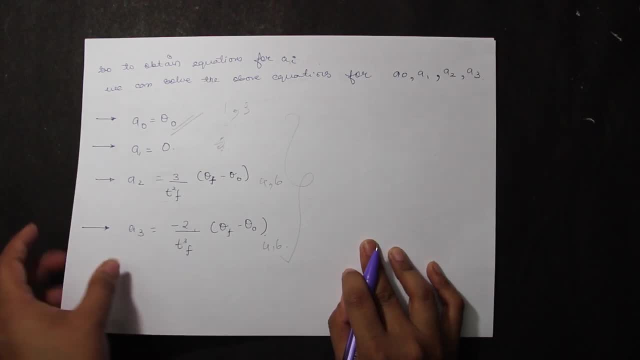 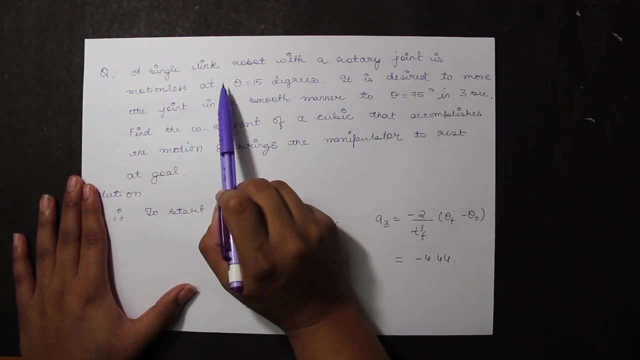 Now let's quickly hop to the next equation, To a question. you can pause the video and read the question. A single link robot with a robot joint is motionless at theta equals to 15 degrees, which means our starting value of theta is 15 degrees. 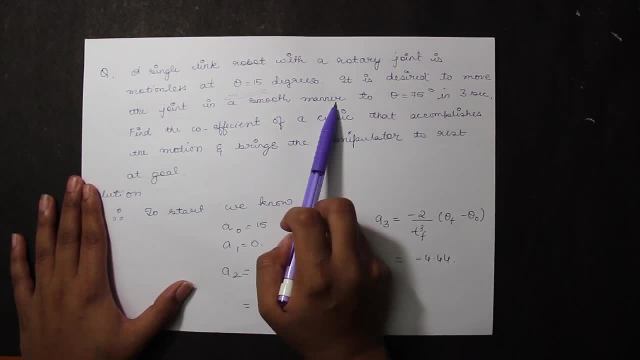 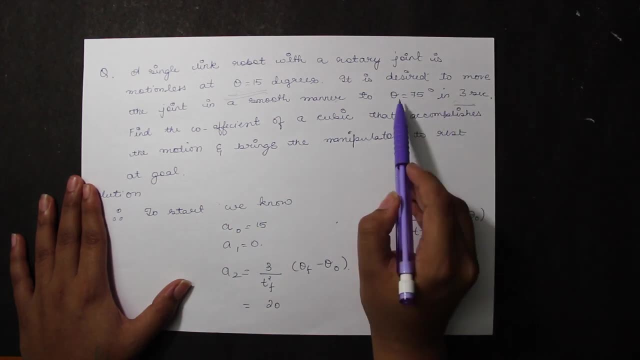 It is desired to move the joint in a smooth manner to. theta equals to 75 degree in three seconds, That is, the time period is three and the theta final, that is, tf of theta, is 75 degree. Find the coefficient of a cubic that accomplishes the motion and brings the manipulator to rest at goal.